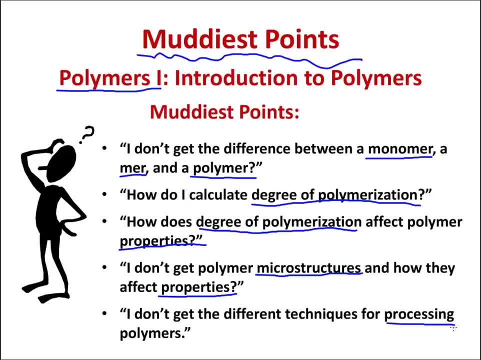 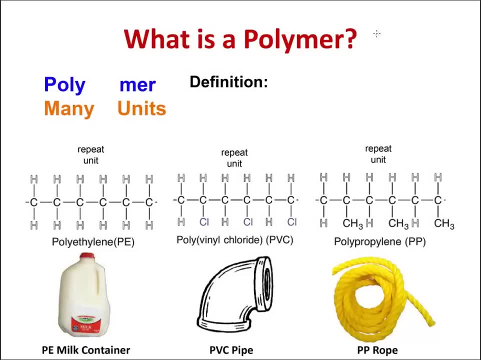 And I don't get the different techniques for processing polymers. If there is a specific topic that you wish to see, there are annotations for the different topics on top of the question mark guy up here. Let's get started Before I begin answering the muddiest points listed on the previous slide. 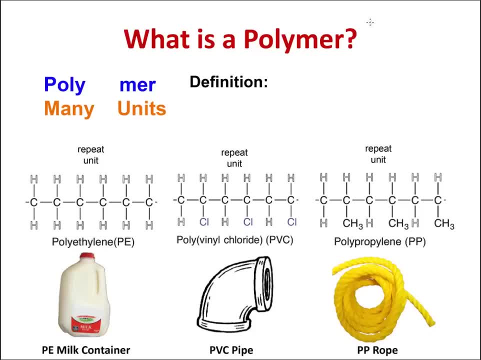 it's important for us to understand what polymers are. You're probably familiar with polymers, because anything that is considered a plastic is a polymer. The word polymer itself comes from Greek and means poly, many mer units, And the definition of a polymer is: 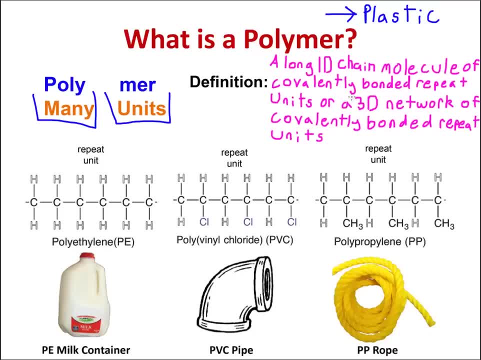 a long 1D chain molecule of covalently bonded repeat units or a 3D network of covalently bonded repeat units. A polymeric solid is a collection of such molecules. Below are three long chain type polymer molecules from everyday life. 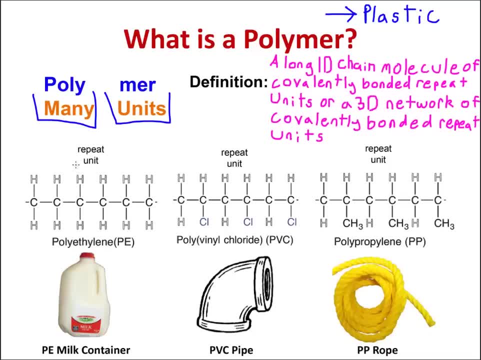 On the far left we have polyethylene, which is used for milk containers, with a repeat unit of chemical composition, C2H4, with the two carbons being main chain carbons. Another polymer from everyday life is polyvinyl chloride, which is used to make PVC pipes. 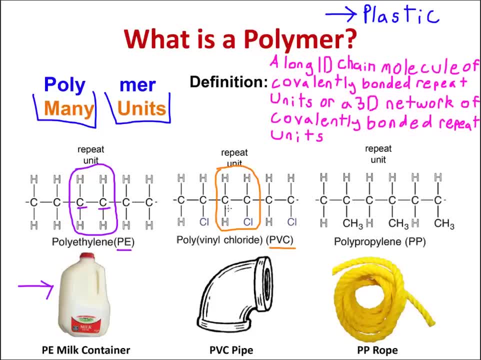 with a repeat unit of C2H3Cl, with the two carbons being main chain carbons. The last polymer that you are most likely familiar with from everyday life is polypropylene, or PP for short. Polypropylene is used for things like polypropylene rope. 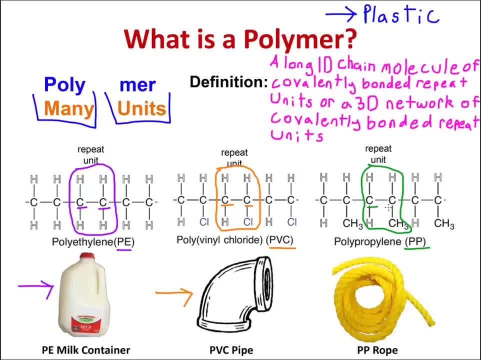 with a repeat unit of C3H6, with two of the carbons being main chain carbons and the third one being part of a side group, CH3.. The three polymers shown have a similar structure, but the main difference is an atom or group attachment. 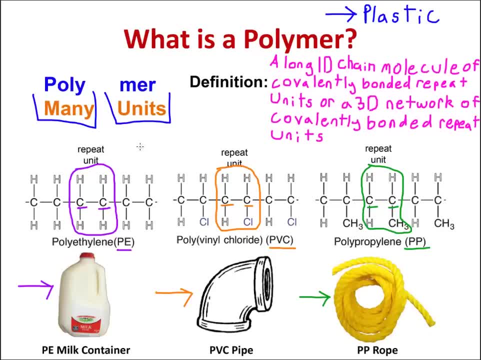 which we refer to as a substituent. For example, there is one substituent that is different for each of these three. example: polymer molecules. In polyethylene, there are four hydrogens. In polyvinyl chloride, there are three hydrogens and then one chlorine substituent. 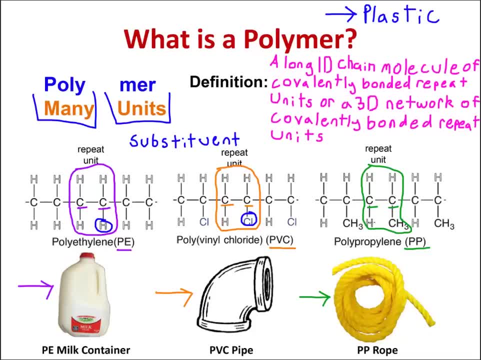 And then for polypropylene, there are three hydrogens and then a CH3 group substituent. So that's the difference. Now, different substituents cause significant differences in structure and properties. But before we get to that, in the next slide we will discuss 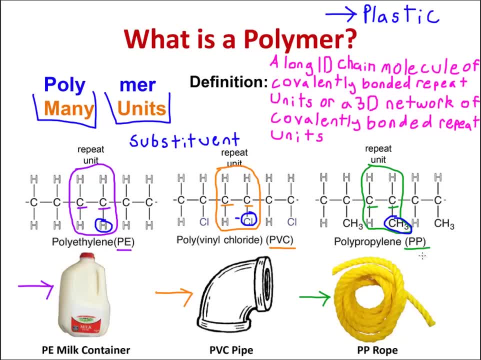 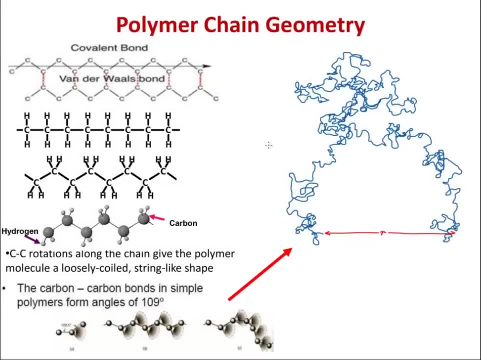 the nature and characteristics of a 1D covalently bonded long chain molecule. On the previous slide I told you that polymers are long chain molecules of covalently bonded repeat units And I also showed you three example polymer chains for common polymers. 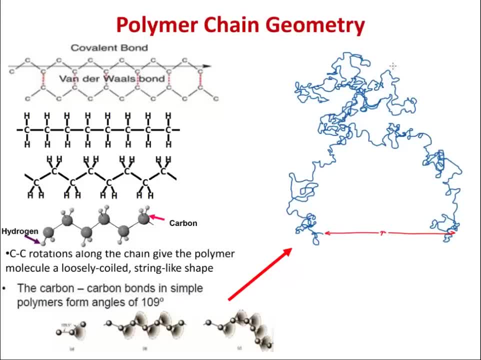 However, those chains didn't tell you what the polymer chain looks like as a whole. So the goal of this slide is to answer the question: what do the example chains we talked about on the previous slide look like as a whole? Well, complete polymer chains. 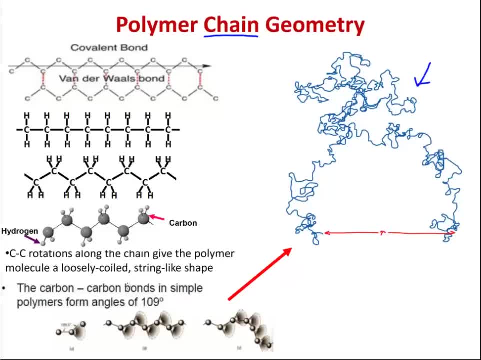 look something like this diagram. here We can see that the polymer chain is loosely coiled and has a string-like shape. This is because the carbon-carbon single bonds rotate to form angles of 109 degrees. Why does this cause a coiled, string-like shape? 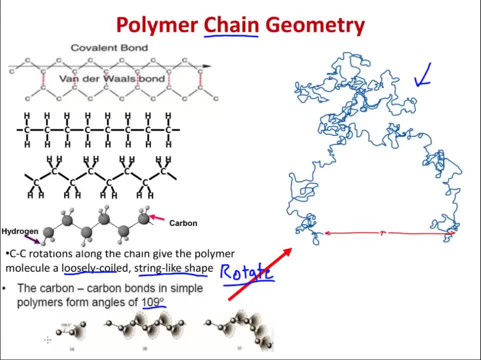 Well, in three-dimensional space there are many different ways to form angles of 109 degrees, as shown by this diagram. here I've included my own rendition of this diagram. We can see that the 109 degree angle is formed here and for this, carbon here. 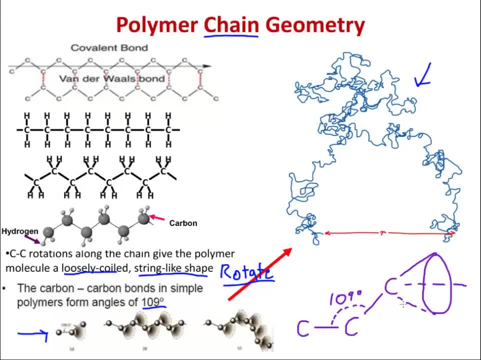 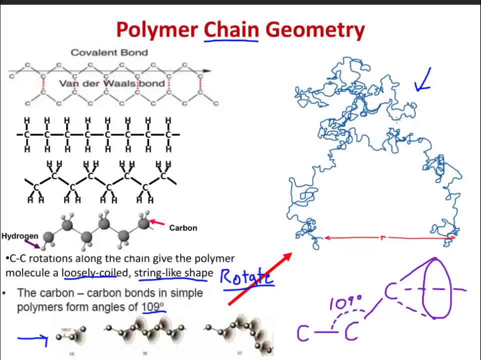 if we placed a bond anywhere on this circle, the bond angle would be 109 degrees And because there are so many single carbon-carbon bonds in the chain, each one forms the 109 degree bond differently. Now that we have an idea of what the polymer chain looks like, 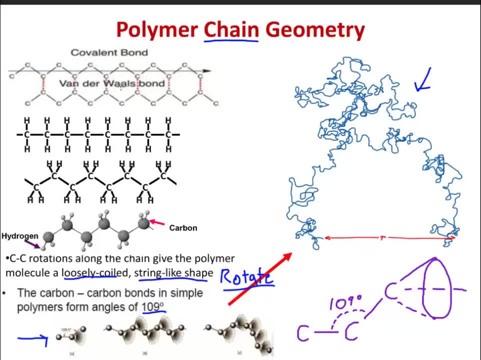 how do the chains interact with each other? Well, between each of the single polymer chains, we have van der Waals bonding, which holds the polymeric solid together as a whole. If you would like some more review about van der Waals bonding, I've included an annotation. 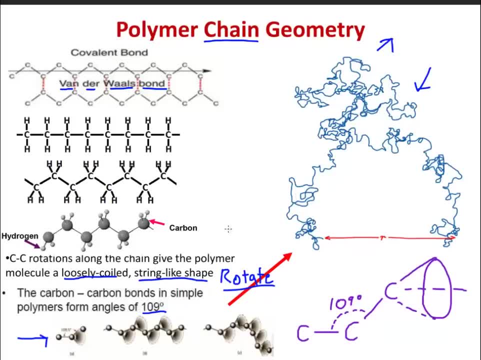 to the bonding video from this channel. Finally, I've also included three representations of polyethylene or PE chains as an example, looking from different viewpoints. This diagram is the view of a polyethylene chain from the top. This view here is polyethylene from the side. 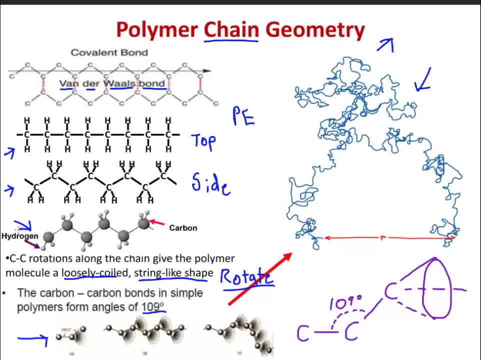 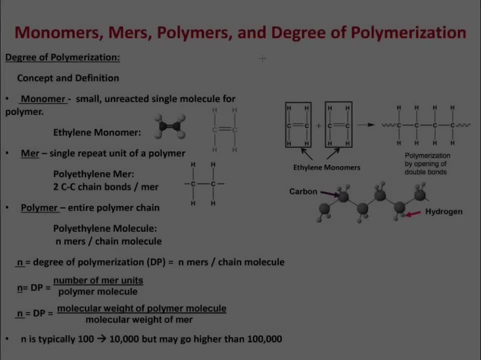 Finally, in this diagram below, we have polyethylene given as a ball and stick model. Again, these three diagrams are not the complete polymer chain. they're just to show you how the polymer molecule looks from different viewpoints. Now that we have a general idea, 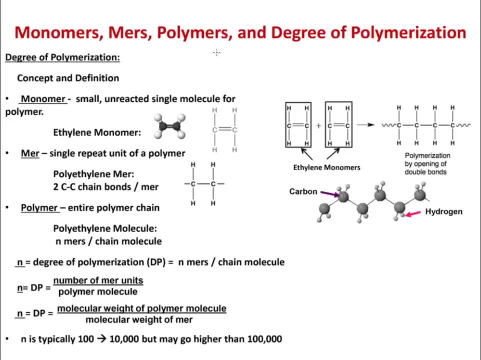 about what polymers are. I can now address the muddiest points concerning the difference between monomers, mers and polymers, and also describe degree of polymerization and do an example calculation for it. So a monomer is a small unreacted. 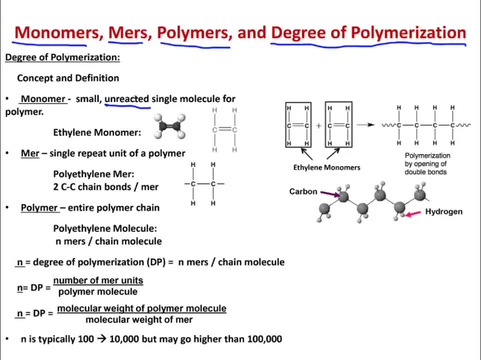 single molecule for the polymer. The keyword here is unreacted. As an example, I'll be using ethylene and then eventually polyethylene throughout this slide. Here are two representations of an ethylene monomer: the ball and stick model here and the Lewis structure here. 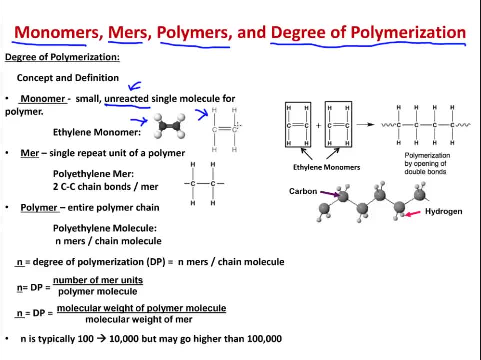 One important thing to note is that there is a double bond between the carbon atoms in the monomer. Now, on the other hand, a mer is defined as the single repeat unit of the polymer. The mer has been reacted, and that is how it's different. 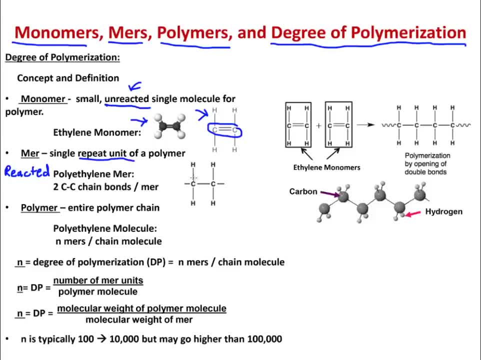 from the monomer, Again using polyethylene as our example. here is what the polyethylene mer looks like. Notice that there isn't a double bond between the carbon atoms, but there is now a single bond. Also, there are two carbon-carbon chain bonds. 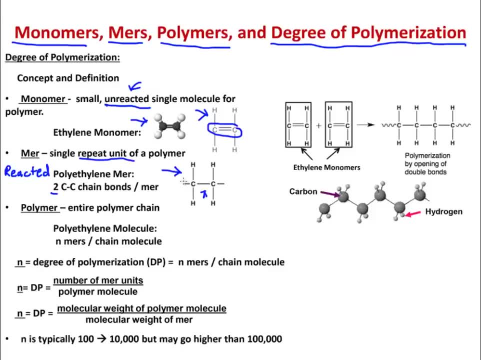 in each polyethylene mer, because on the left we have one half of a bond between the two carbons, here we have a whole bond And on the right here we have half of a carbon-carbon single bond. To further emphasize the difference between monomer and mer, 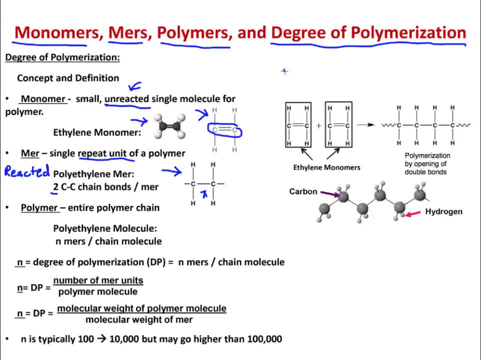 I've included a simple diagram above. Here is before the reaction occurs. you've got two ethylene monomers and then a chemical reaction called polymerization occurs, which will be talked about in a later video. After the polymer has been polymerized, the former monomers are now incorporated. 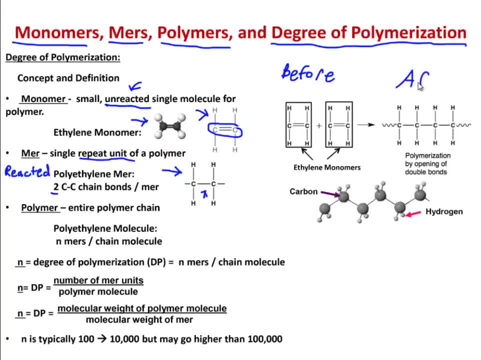 into the linear 1D chain of single carbon bond mers for polyethylene that I'm using for an example, So there would be a mer here and here. Finally, I've already discussed what a polymer is, but to review the polymer refers to the entire. 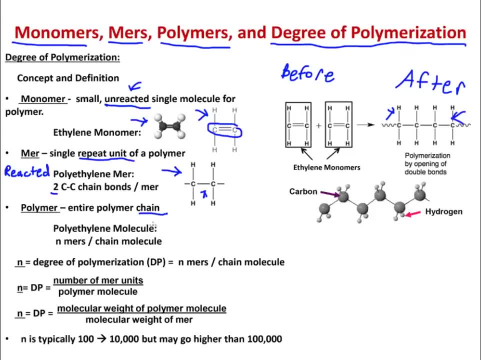 chain molecule. Okay, So we've defined monomer, mer and polymer. Now we can speak about the concept of degree of polymerization, which is defined as the number of mer units per polymer molecule. It is abbreviated by a lowercase n most of the times. 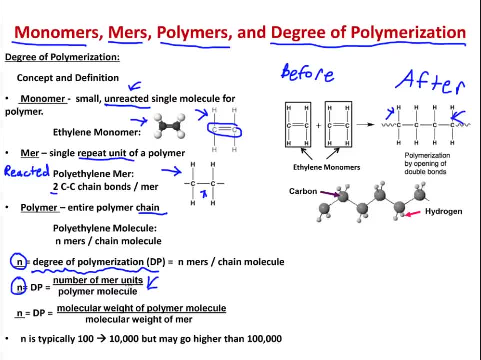 So n degree of polymerization is defined as the number of mer units per polymer molecule. Now there is a shorthand way that is commonly used to represent an entire polymer chain that involves the degree of polymerization. So if we know the mer and we know the degree of polymerization, 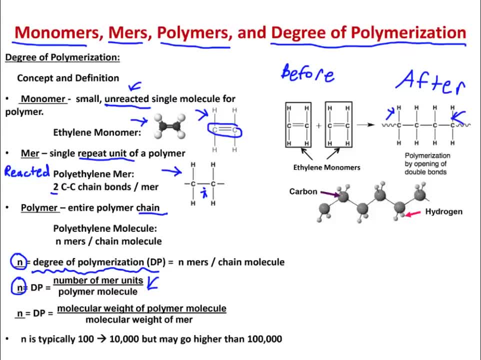 we can represent the entire polymer chain by using the following notation. I'm going to erase this and this. Alright, If we know the mer unit, we can put it in parentheses like so, parentheses like that, and then put n at the bottom right hand corner. 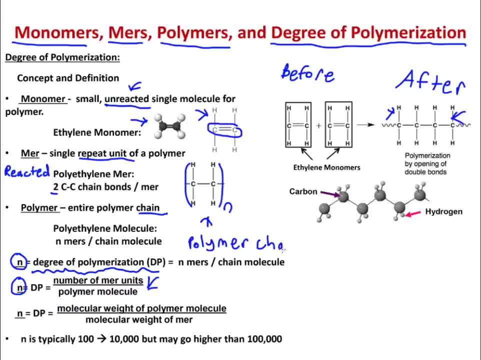 to represent the entire polymer chain, And this is how you usually see polymer chains written out in textbooks. Another way that we can find the degree of polymerization n is by the formula: the molecular weight of the polymer molecule divided by the molecular weight of the mer. 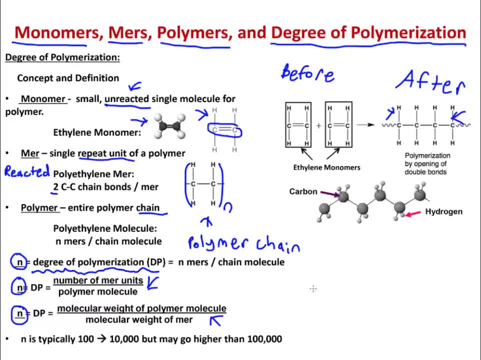 which makes sense. Let's do an example. problem with degree of polymerization. Let's pretend that I'm looking for the molecular weight of a polyethylene molecule and I know that the degree of polymerization n is 1000.. How can I find the molecular weight? 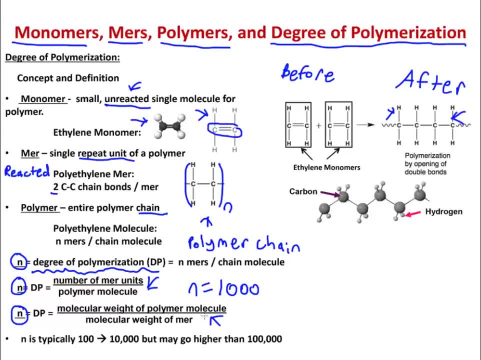 of the polymer molecule. I can rearrange this equation to solve for the molecular weight of the polyethylene molecule. so n times the molecular weight of the polyethylene mer is equal to the molecular weight of the entire chain. So now I already know n how do I find the molecular weight of the mer? 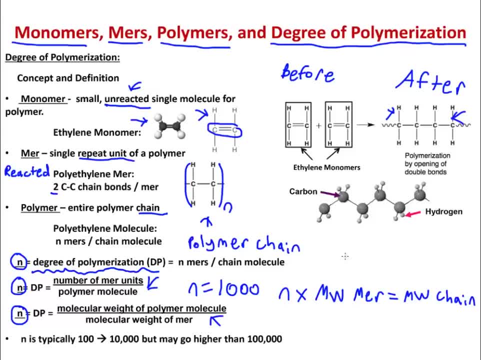 I first have to know what the mer is, which is given here. Using a periodic table, we can look up that the atomic weight of carbon is 12.01 grams per mole and the atomic weight of hydrogen is 1.01 grams per mole. 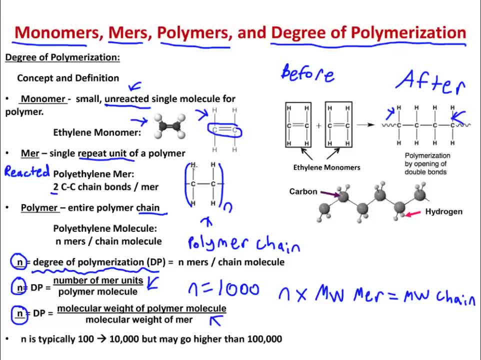 So 4 hydrogens 4 times 1.01 grams per mole, plus 2 carbons 2 times 12.01 grams per mole, gives us that the molecular rate of the mer would be 28, .06 grams per mole. Now plugging in our 1000, 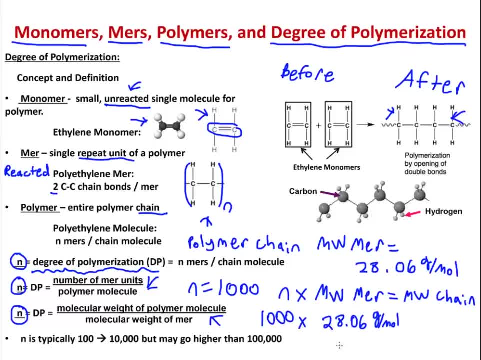 and our found molecular weight of the mer, we can see that the molecular weight of the chain would then be 28,060 grams per mole, And that's just a very easy example of how we can use degree of polymerization As a side note. 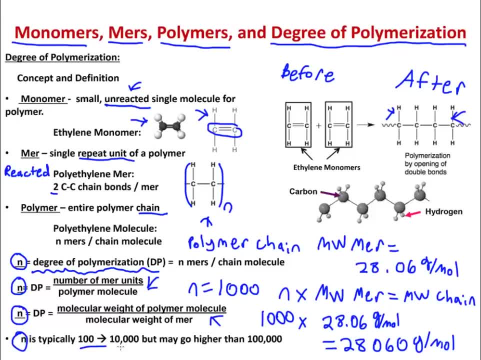 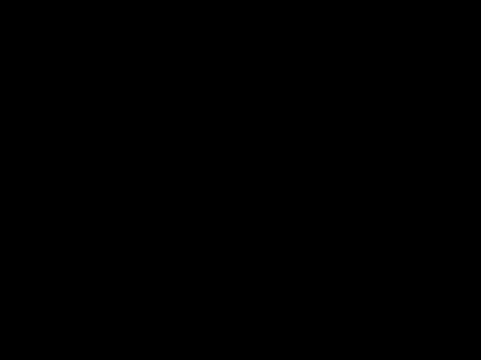 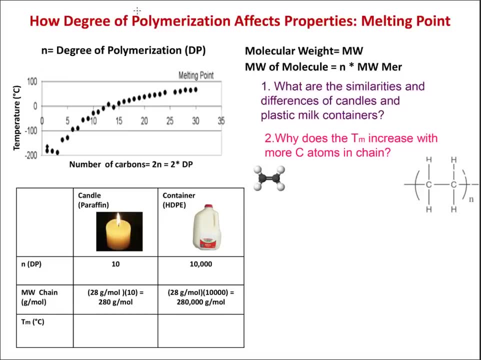 the degree of polymerization n is typically 100 to 10,000, but may go higher than 100,000 depending on the circumstances. On the previous slide, terminology related to polymers was discussed. One of the discussed terms was degree of polymerization. 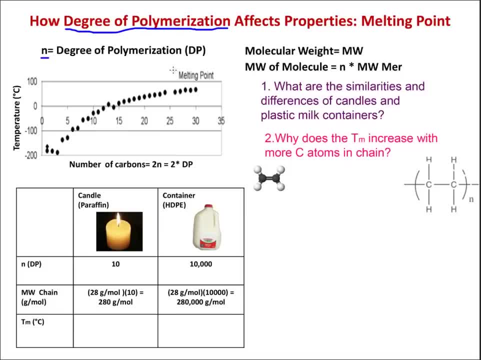 Now the degree of polymerization is abbreviated by lowercase m and is related to the molecular weight of the molecule and the molecular weight of the mer. according to this equation Now on the previous slide, the degree of polymerization may have seemed a bit abstract. However. degree of polymerization. 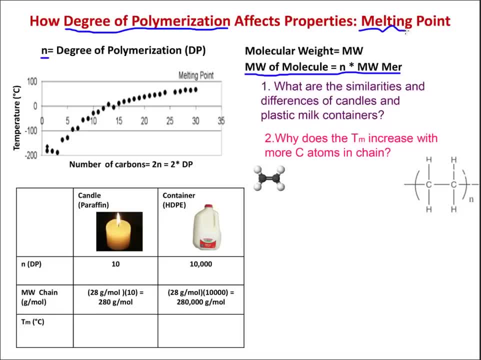 affects properties that are important, such as the melting point of the polymer, And in order to demonstrate this, I will be comparing two everyday items: A candle which is made of paraffin and a milk container which is made of high density polyethylene, or HDPE. 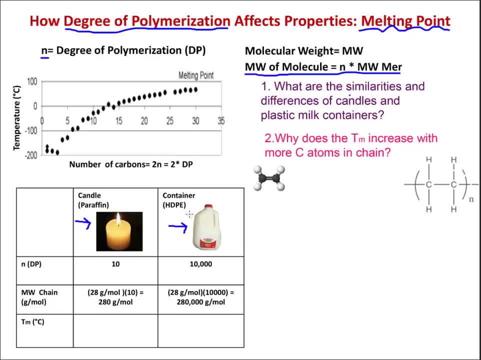 One of the similarities between paraffin and HDPE is that they can both be written this way in polymer notation shorthand, where n stands for the degree of polymerization and the mer is in the parentheses here. So paraffin and HDPE both have the same. 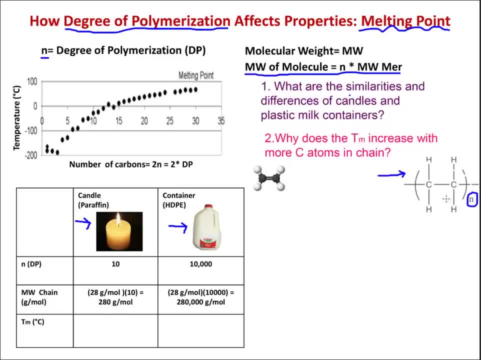 mer, which is ethylene. What are some of the differences between paraffin and HDPE? Well, paraffin has a degree of polymerization of 10 and HDPE has a degree of polymerization of 10,000, which is way, way, way bigger. 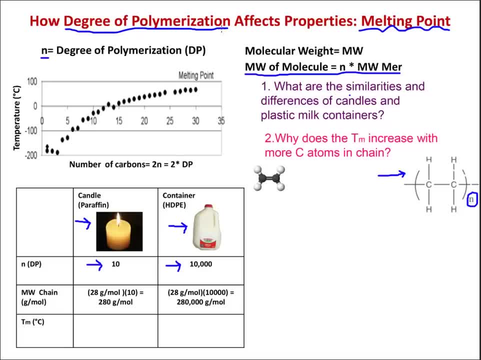 The molecular weight of a chain of paraffin can be found using this equation here and using the fact that this ethylene mer weighs 28 grams per mole, as determined on the previous slide. So the molecular weight of a paraffin chain would be 28 grams per mole. 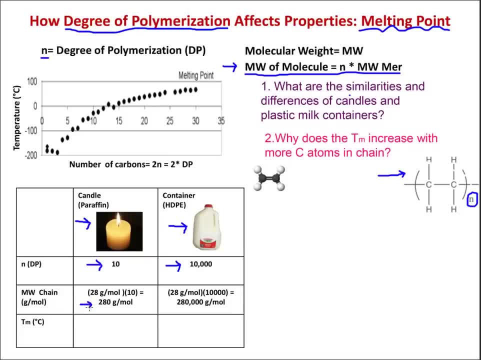 times 10 or 280 grams per mole. Doing a similar calculation with HDPE, we can see that the molecular weight of an HDPE chain is much greater, at 280,000 grams per mole. But how does this affect your melting temperature? Well, 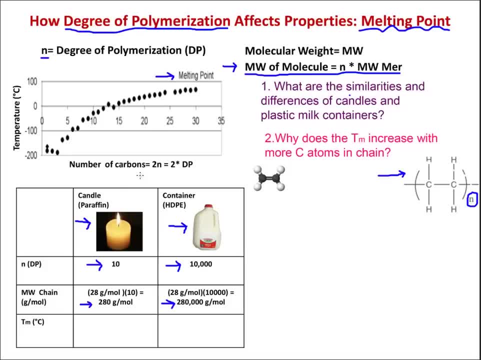 right here I have a graph that gives me a melting point with number of carbons on the x-axis and temperature in degrees Celsius on the y-axis. So in order to find the melting point in degrees Celsius, I need to know the number of carbons in the 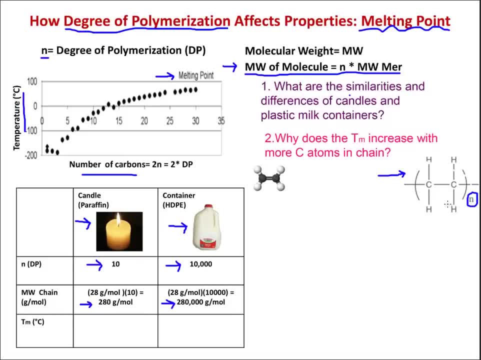 chain For polymers. with this mer the number of carbons in the chain would be 2 times the degree of polymerization. So for paraffin the number of carbons in the chain would be 2 times 10 or 20.. So we can find the. 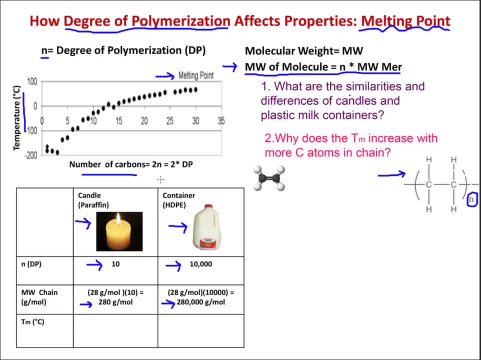 melting point of paraffin using this graph. So going to 20 carbons in the chain on the x-axis and then reading up to the curve which represents melting point, and then reading over to the y-axis, will give us our melting point for paraffin. 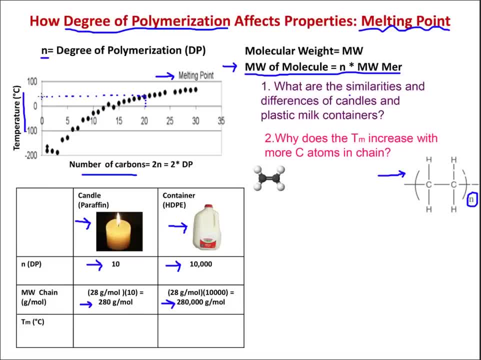 We can see that the melting point of paraffin is about 40 to 50 degrees Celsius. The number of carbons in an HGPE chain would be 2 times 10,000 or 20,000, which is not shown on this graph here. 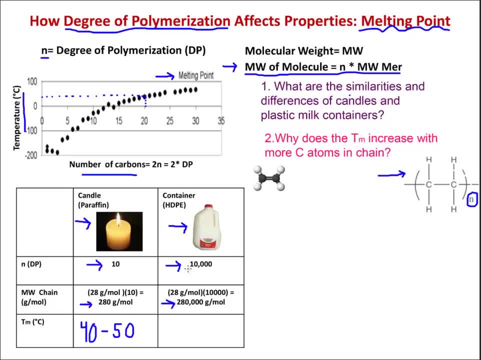 on the x-axis, So we can't find that using this graph. However, the melting point of HGPE levels off at a certain point, So the melting temperature of HGPE is about 120 to 130 degrees Celsius. So, in summary, as N increases. 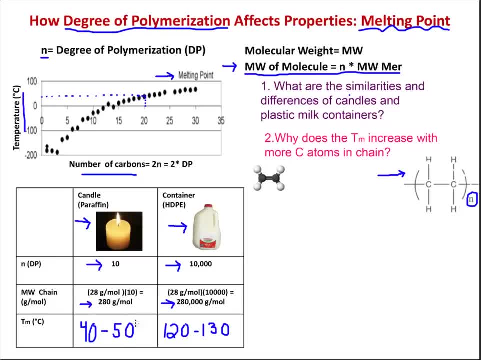 so does the molecular weight of the chain and in general, so does the melting point. But the million dollar question is: why does the melting temperature increase with more carbon atoms in the chain? Well, let's think about what governs the melting temperature in a linear 1D polymer. 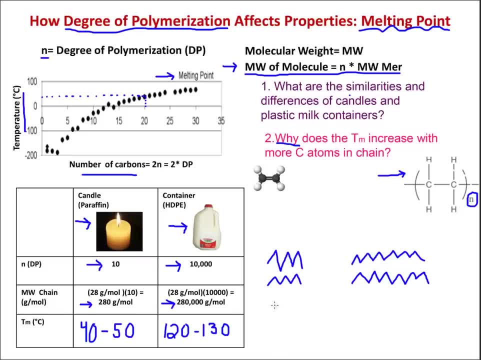 Well, in a linear 1D polymer, the melting point is determined by the amount of van der Waals bonding in the polymer, because that is what holds the polymer solid together as a whole and what holds the chains together. So in a polymer with a high degree of polymerization, 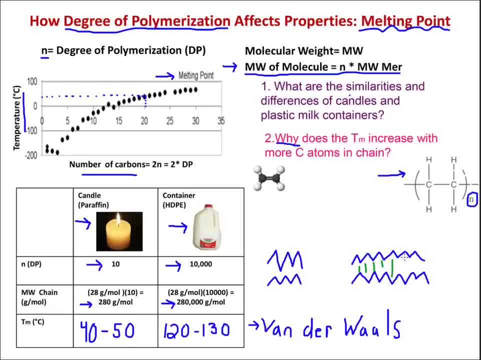 as in the picture on the right that I'm putting van der Waals bonds in green in. now this polymer has more van der Waals bonds in it than one with a lower degree of polymerization on the left. So this one, the one with the higher N, 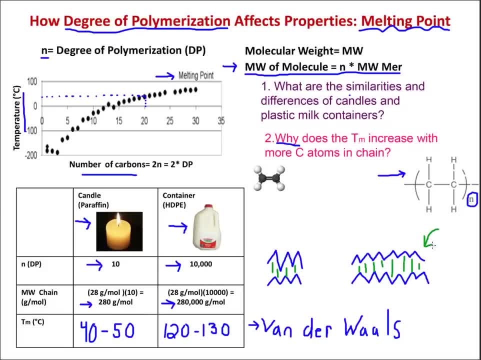 has more van der Waals bonds which need to be overcome to melt, so this one has the higher melting temperature So far. the only kind of polymer that has really been discussed are 1D linear polymers. Now this polymer type is called thermoplastic. 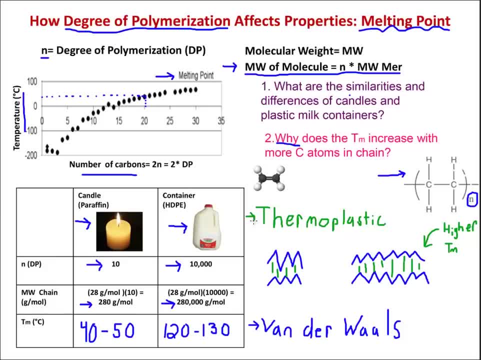 And this term will be defined later on, but thermoplastic polymers are one of two main types of polymers, And the next few slides are going to focus on how we can categorize these polymers based off of their internal structures and how those 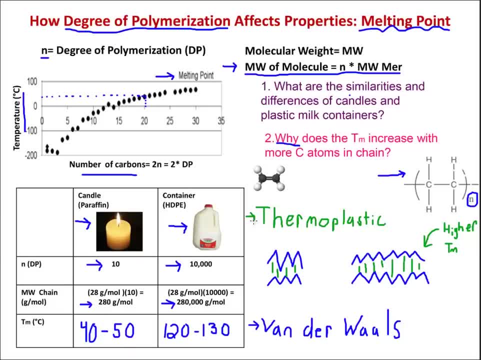 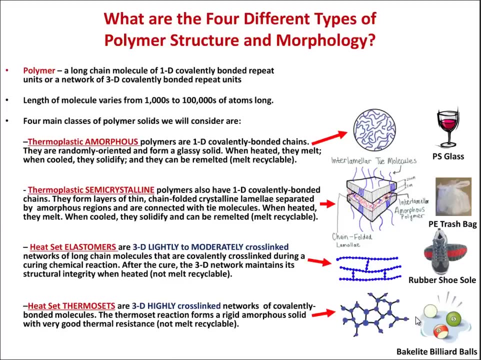 internal structures affect macroscopic properties like tensile strength, elastic modulus- things that are important to us. The primary type of polymer that has been focused on in this video up to this point is 1D linear polymers. However, there are more types of 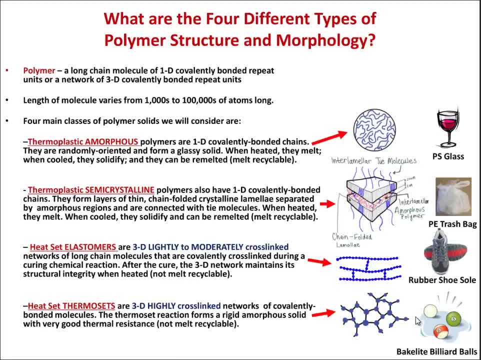 polymers than just that. The 1D linear polymers that have been discussed up until this point are under the category of thermoplastic, which means that they can be melted and remelted. However, on the other hand, there are also heat set. 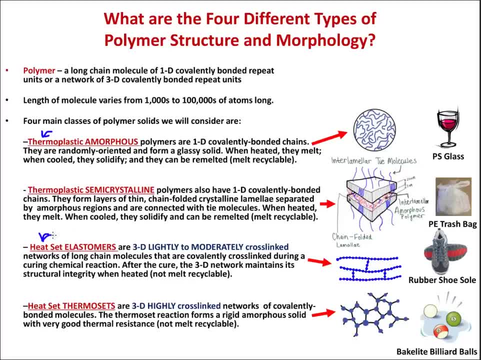 polymers, which means that once they're heated they react to form a 3D covalently bonded network And the shape of the material is permanent and will not melt if it is heated. From those two main classifications of polymers- thermoplastic and heat set- 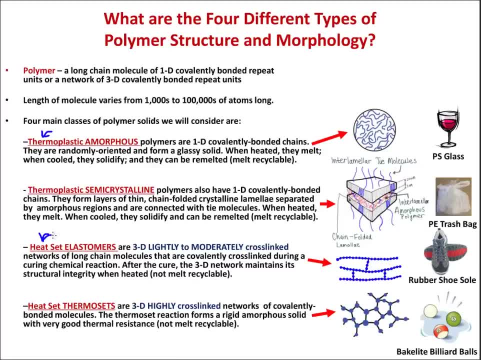 there are four main ways that polymers organize themselves. There's an easy way to classify these polymers: based on their internal structure, and it's important to note that this internal structure controls macroscopic properties we care about. So there are four main types of polymer structure. 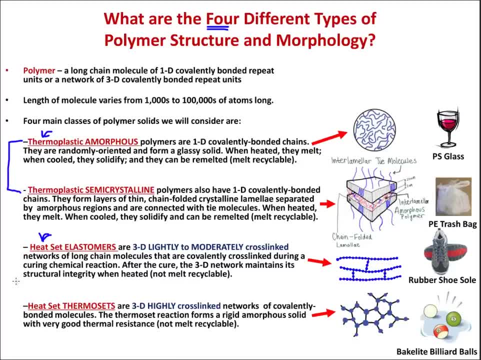 under the two main categories of thermoplastic and heat set. Under the category of thermoplastic, we have thermoplastic amorphous polymers. They are 1D covalently bonded chains. They are randomly oriented and form a glassy 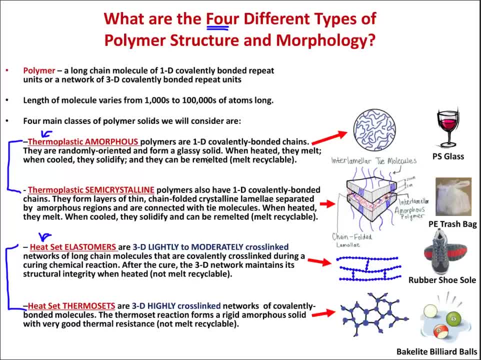 solid. When heated they melt. when cooled, they solidify and they can be remelted because they're thermoplastic. The microstructure of a thermoplastic amorphous polymer looks like this: No organization in here: An everyday item made of a thermoplastic. 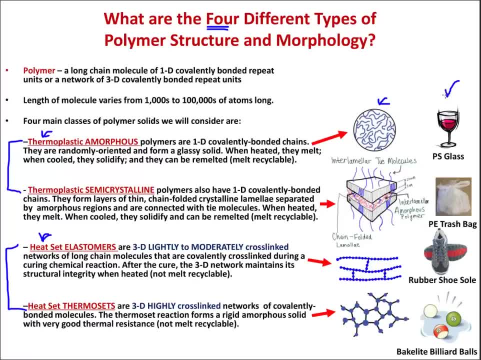 amorphous polymer would be a polystyrene wine glass. Also under the thermoplastic category of polymers we have semi-crystalline polymers. They also have 1D covalently bonded chains. They form layers of thin chain folded. 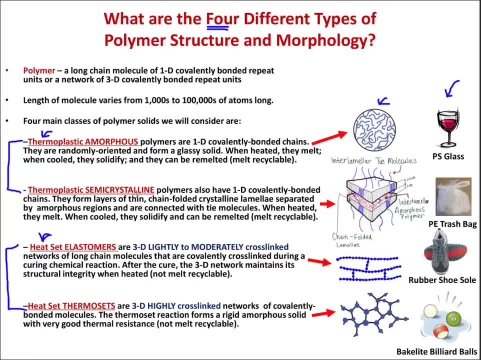 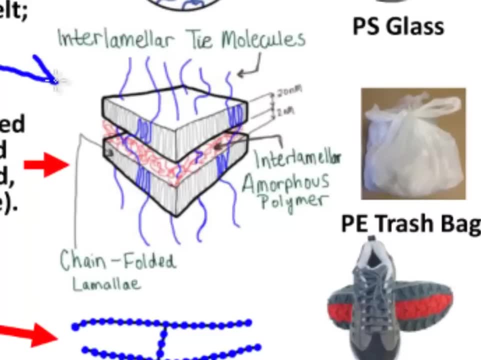 crystalline lamellae, separated by amorphous regions and are connected with time molecules. Again, as all thermoplastic polymers, when heated they melt and can be recycled. Here is what the thermoplastic semi-crystalline microstructure looks like. 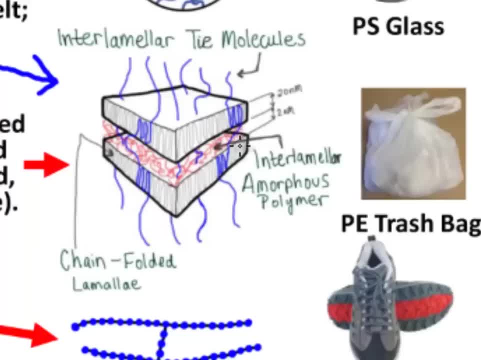 The chain folded lamellae are shown here, and the interlamellar amorphous polymer is here in red, and your time molecules are in blue. An example of an everyday item made with a thermoplastic semi-crystalline polymer would be this: polyethylene. 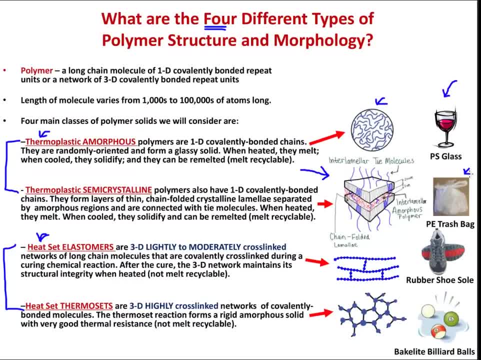 trash bag. Moving on to the second main category of polymers, the heat sets. One type of heat set polymer is elastomers. They are 3D, lightly to moderately cross-linked networks of long chain molecules that are cross-linked during a curing chemical reaction. 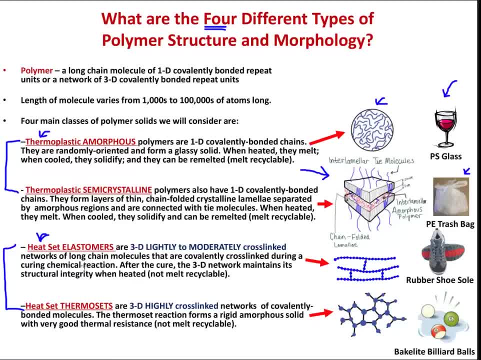 After the cure. the 3D network maintains its structural integrity when heated, and therefore heat set. elastomers are not melt, recyclable. One word that may be unfamiliar to you is cross-linked or cross-linking. Basically, cross-links are covalent bonds that 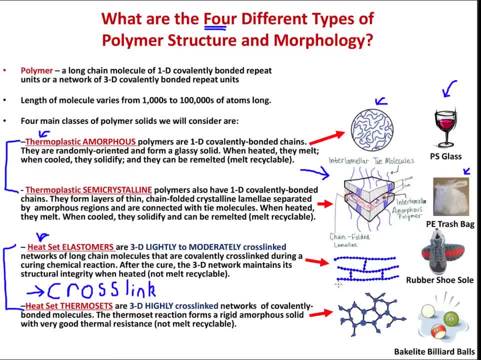 connect chains In the drawn structure of the heat set elastomer microstructure. here these things in the middle would be cross-linked, like here and here and here. Cross-links are one of the important things that define heat set polymers. It is important. 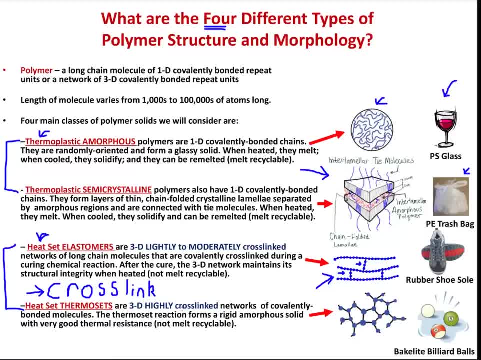 to understand what they are. In a future video we will talk about how cross-linking happens. An everyday item that is made of a heat set elastomer would be the rubber sole of a running shoe. Finally, the fourth main morphology type would be: 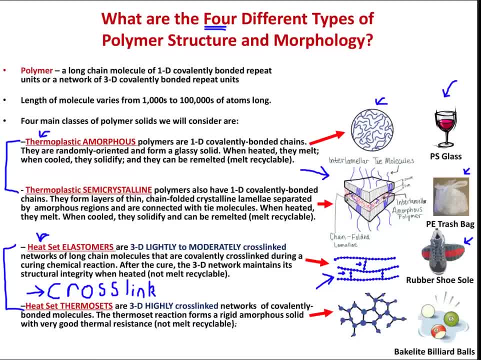 your heat set thermosets. They are 3D highly cross-linked networks of covalently bonded molecules. The thermoset reaction forms a rigid, amorphous solid with very good thermal resistance. This is also not melt- recyclable, If you look. 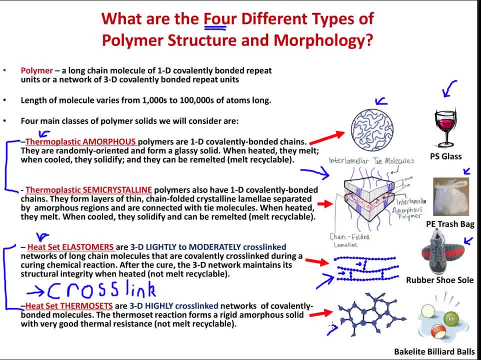 at the structure of a thermoset as shown here, you can see that the network is cross-linked. An example of an everyday item made of a thermoset type polymer would be bakelite billiard balls. To summarize, there are two main types. 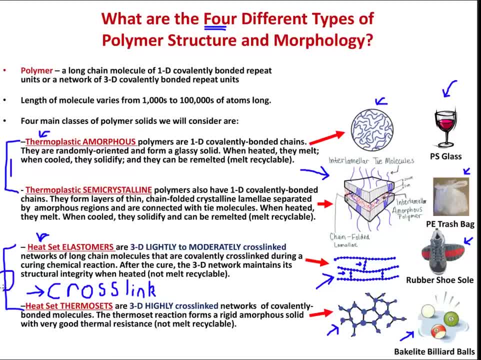 of polymers: thermoplastic and heat set. In the main category of thermoplastic, we have thermoplastic amorphous and thermoplastic semi-crystalline. In the main category of heat set, we have heat set elastomers. 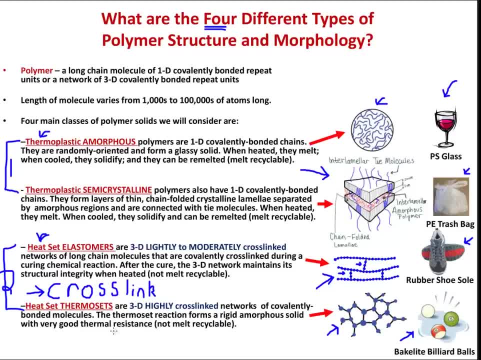 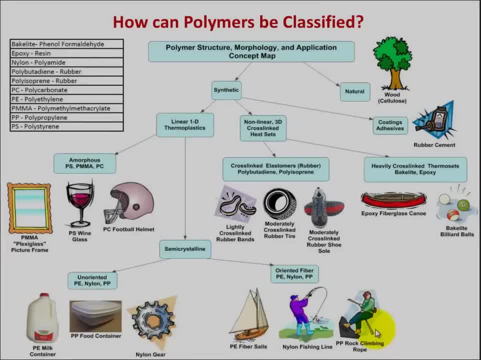 And heat set thermosets. Throughout the rest of the video, we'll be comparing and contrasting between the four main polymer structures and morphologies, Now that the four main morphology types of polymers have been discussed: thermoplastic, amorphous, thermoplastic, semi-crystalline. 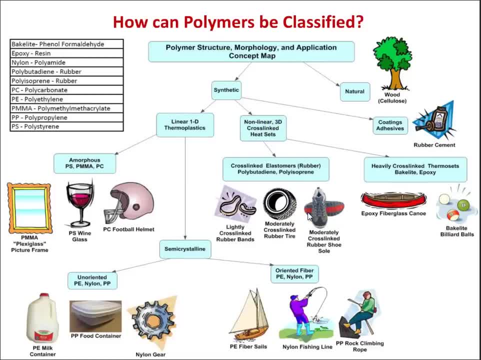 heat set elastomers and heat set thermosets. this serves to show the relationships between the polymer types and to also give some more everyday examples of each different type of polymer. In order to read this concept map, you start at the very top and 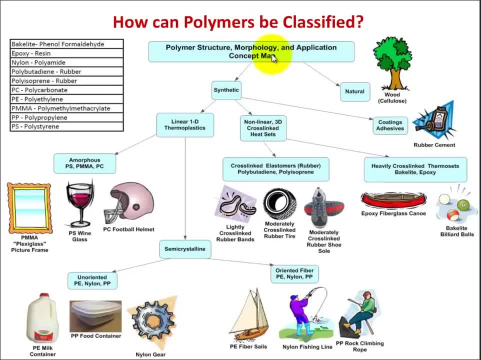 read down following the arrows. So, for example, under polymers in general, we have our natural polymers, like wood, and synthetic polymers, And then, under the category of synthetic polymers, we have linear 1D, thermoplastics, 3D, crosslinked heat sets. 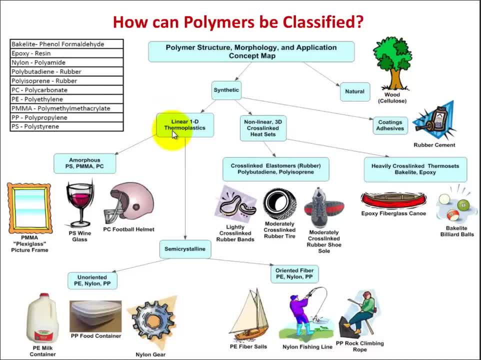 and coatings and adhesives, And then, under linear 1D thermoplastics, you have your amorphous or semi-crystalline. A later video will talk about high performance oriented polymer fibers. These fibers consist of long covalently bonded polymer. 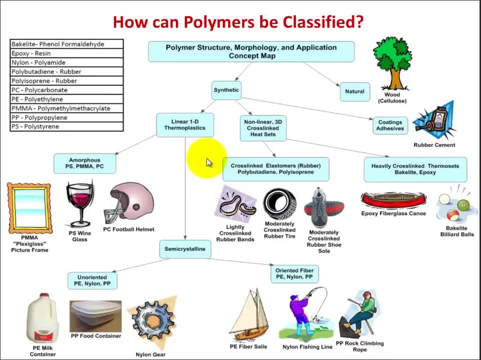 chains oriented in a single direction, giving them high strength and stiffness. This video talks about unoriented polymers. only Then, under your 3D crosslinked heat sets, you've got your elastomers and your thermosets. So this slide again just serves to. 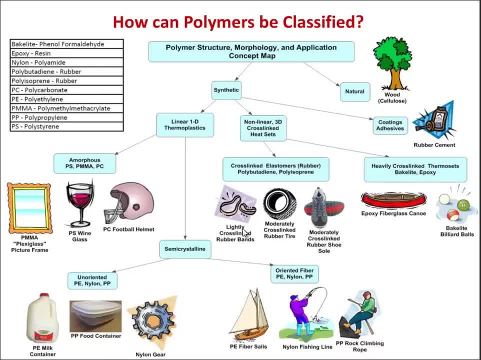 give a visual of how polymers can be classified. As a final note, the abbreviations like PMMA would be polymethyl methacrylate, and what each of the abbreviations mean is found in this box up here. So now that the big picture of how polymers 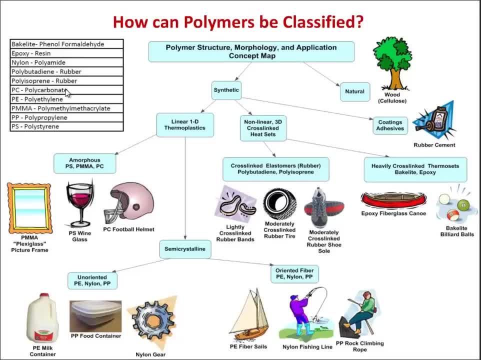 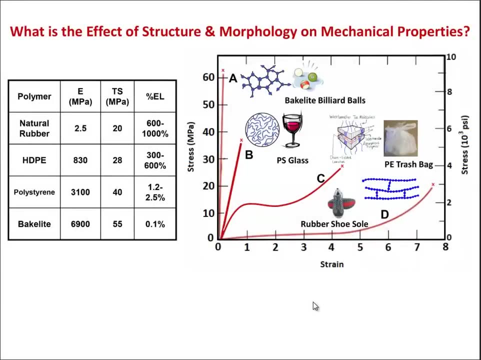 are classified has been discussed. the next few slides are going to be about how do these morphologies and structures affect properties that we care about and how we process these different types of polymers. We've already talked about the four different types of polymer morphologies. 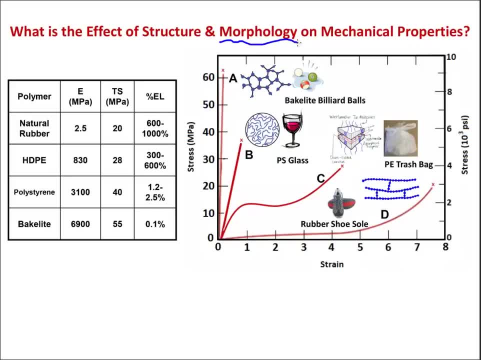 but how do those morphologies affect mechanical properties that we care about, like elastic modulus, tensile strength and percent elongation, which is ductility For all the materials except for rubber, which it's more of a percent elasticity measurement? here I have four curves. 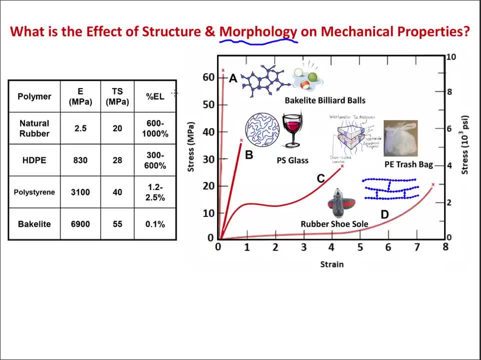 representative of the four types of polymers. But before I begin, it's important to bring up a thermal property that hasn't been discussed yet, So I can explain these four different behaviors. Polymers are unique because they have this thermal property called the. 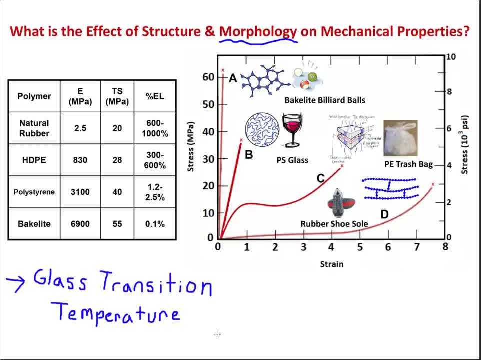 glass transition temperature. Basically below this glass transition temperature, the amorphous regions of the polymer behave prettily and glassy. and above this glass transition temperature, the amorphous regions of the polymer act like a very viscous liquid which is leather-like. 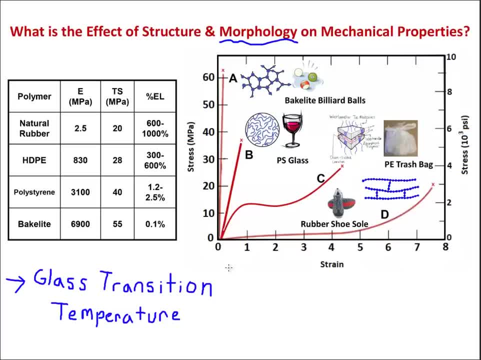 So the glass transition temperature is defined as the temperature at which the amorphous regions of a polymer upon cooling goes from being a viscous, leather-like liquid to being a brittle, glassy solid. As you can see, I have a stress-strain curve. 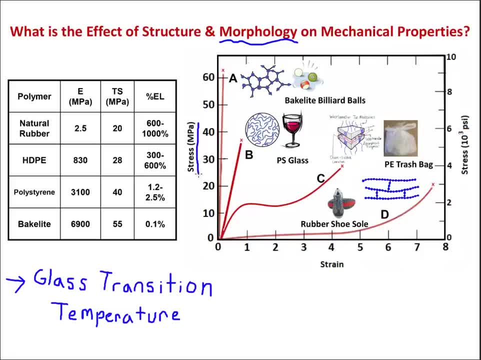 here with stress and MPA on the y-axis and strain on the x-axis. I will now go through and match each polymer with its mechanical properties and explain why they are that way. So to begin with, curve A is representative of heat-set thermoset polymers. 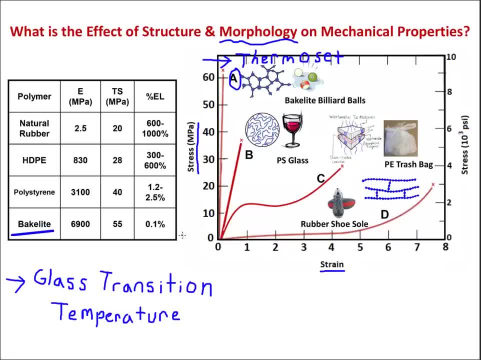 Curve A here is bakelite And, as we can see, its elastic modulus is the highest of the four. Its tensile strength is also the highest of the four. However, its ductility is the lowest. Why is that? Well, as you can see by the morphology, 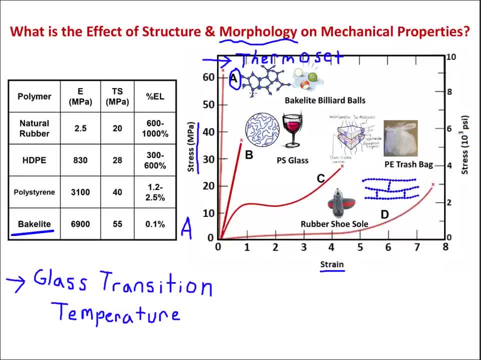 this thermoset is a net and is made strong by its cross-links. Also, it's important to note that all of these stress-strain curves were taken at room temperature, so about 25 degrees Celsius. So at 25 degrees Celsius, bakelite. 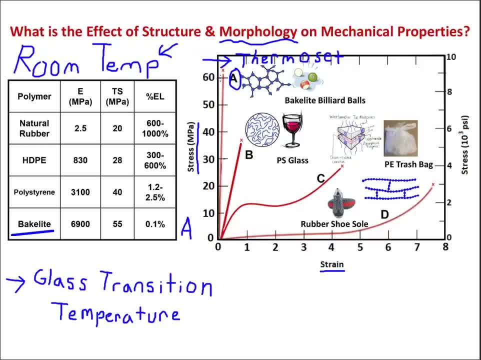 is below its glass transition temperatures, which is why you see its stress-strain curve behaving in a brittle manner. Curve B: here is polystyrene, representative of thermoplastic amorphous polymers. As you can see, polystyrene is. 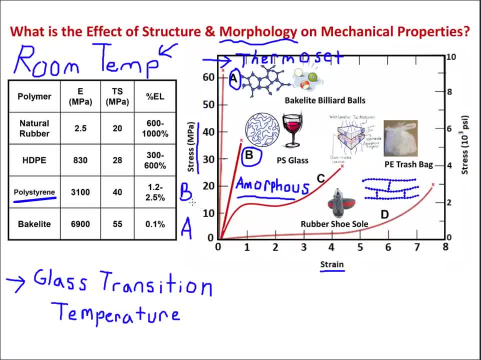 the second highest elastic modulus, second highest tensile strength and second lowest ductility. And polystyrene at room temperature is also below its glass transition temperature, so it is also behaving as a glassy solid, as seen by the brittle behavior of the. 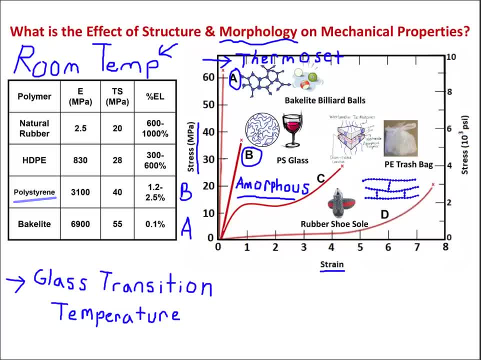 stress-strain curve, though it does not have cross-links structure. The van der Waals bonding and the amorphous structure make it stronger than curves C or D. Curve C is representative of thermoplastic semi-crystalline polymers. 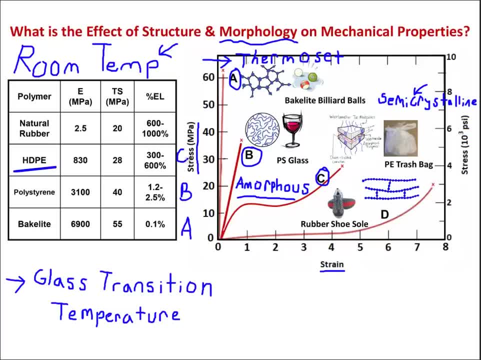 It is of HDPE and, as you can see, it has the third lowest elastic modulus, third lowest tensile strength and third highest ductility. Why is this? Well, at room temperature. the thermoplastic semi-crystalline polymer. 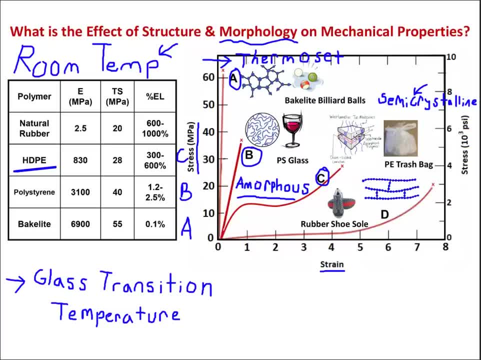 is above the temperature at which the semi-crystalline regions would melt, but below the glass transition temperature of the amorphous regions. So that's why you get this intermediate type of behavior. Finally, curve D is representative of heat-set elastomers. 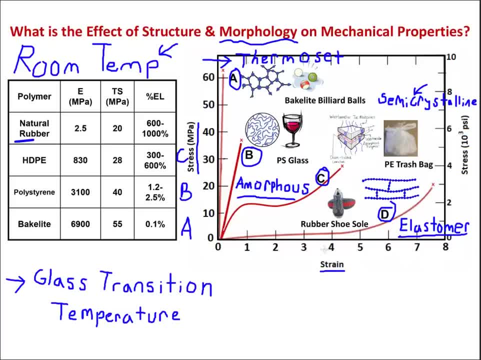 The material shown here is natural rubber and, as we can see, natural rubber has the lowest elastic modulus, lowest tensile strength, but highest ductility. and this is because elastomers at room temperature are above their glass transition temperature. So, without these cross-links between 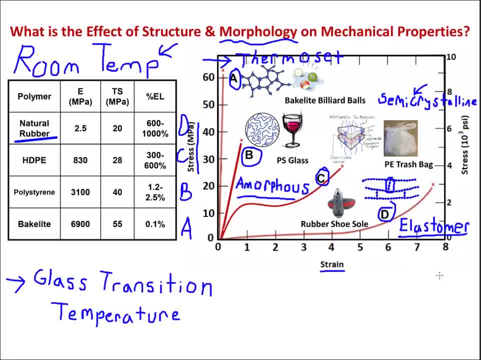 the chains. the elastomer would be a viscous, liquid, gooey mess, But because of the cross-links it can at least be a solid. So there you have it: four curves representative of the four morphology types, Along with an explanation. 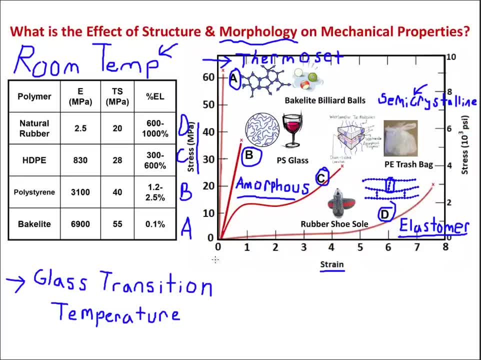 of their mechanical behavior, based off of this thing called the glass transition temperature and their microstructure. So on the next slide I'll go a little bit into more depth of the glass transition temperature and compare and contrast these polymers. just a little bit more for clarity. 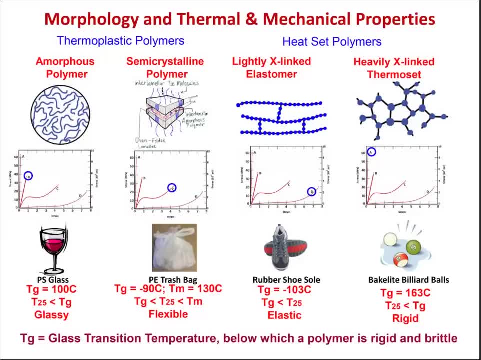 We've already discussed how a polymer's morphology affects some of its mechanical properties, and we've talked about this idea of a glass transition temperature Below which the amorphous regions of a polymer is rigid and brittle and above which the polymer is viscous. 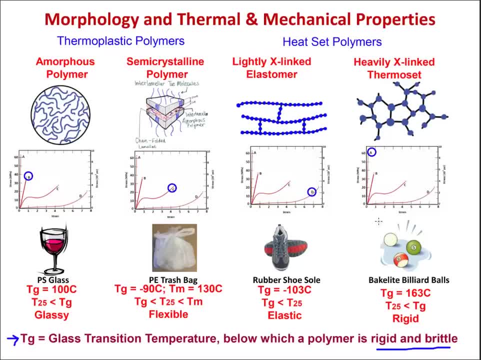 and leathery. The goal of this slide is to organize the information that we've already gotten into the categories that have already been discussed in this video. Recall that we have two main types of polymers: thermoplastic polymers, which can be melted, and. 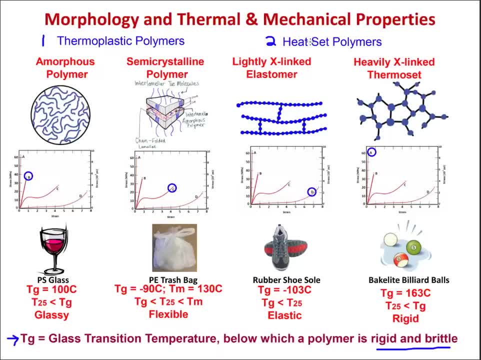 remelted, and two heat-set polymers which, upon curing, they are set during a chemical reaction. So under the category of thermoplastic polymers, recall that we have amorphous and semi-crystalline polymers. Amorphous polymers: 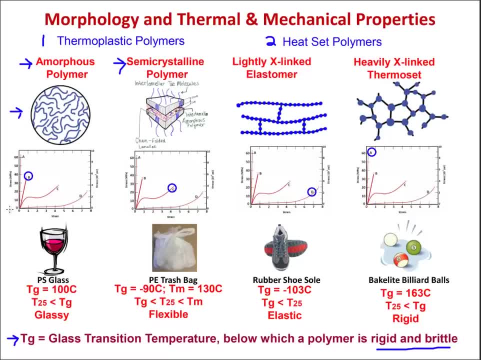 have a microstructure that looks like this and at room temperature, its stress-strain behavior is like this. so it is behaving brittly, as you can see, which is also exemplified in our everyday item, polystyrene glass. 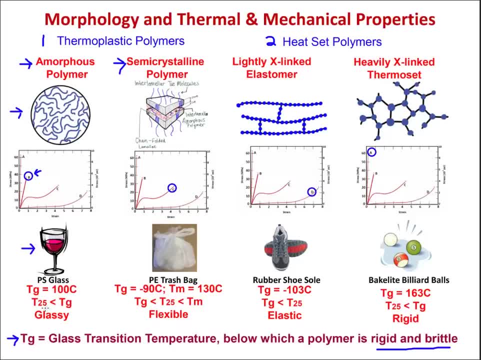 for drinking. Its glass transition temperature is 100 degrees Celsius, so room temperature is far below its glass transition temperature. As expected, polystyrene at room temperature behaves like a glassy and rigid solid. Also under the category of thermoplastic, we have 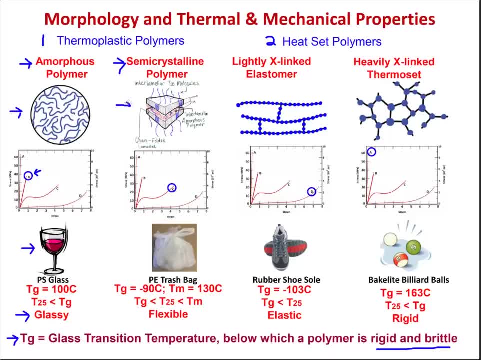 semi-crystalline polymers who have a microstructure that looks like this, a stress-strain curve at room temperature that looks like this, so kind of intermediate because of the two different types of regions, and it's got a glass transition temperature. 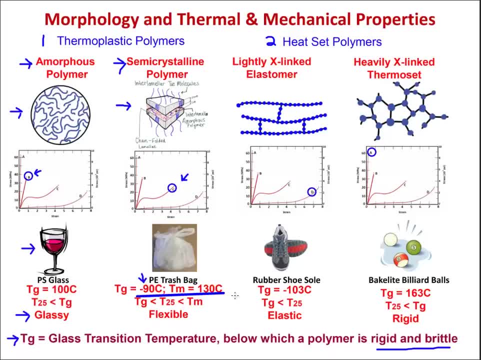 of negative 90 degrees C and its melting temperature is 130 degrees Celsius. So its glass transition temperature is below room temperature and room temperature is below its melting temperature. So therefore, polyethylene, as exemplified by this polyethylene trash bag. 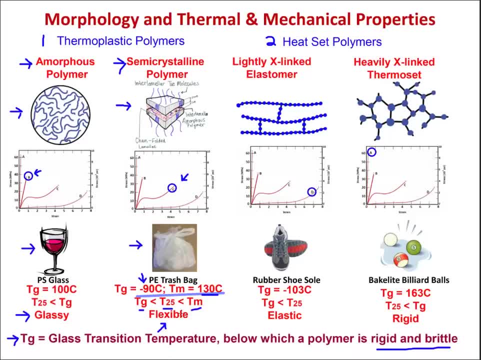 is flexible at room temperature. Finally, moving on to our heat-set polymers, we have lightly cross-linked elastomers and heavily cross-linked thermosets. Lightly cross-linked elastomers have a microstructure that looks like this: a stress-strain curve that looks 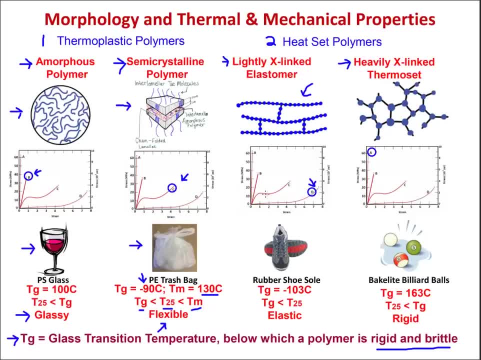 like this and our everyday material would be rubber, as in the rubber in your shoes. Rubber's glass transition temperature is at negative 103 degrees C. Room temperature is way above the glass transition temperature of rubber, so therefore at room temperature. 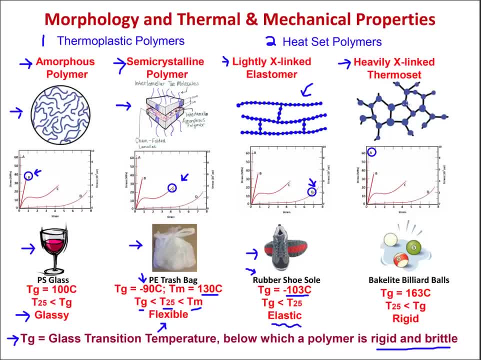 rubber is elastic. Finally, we have our heavily cross-linked thermosets with a microstructure that looks like this and a stress-strain curve that looks like this, which is very brittle. The material we've been using as the example thermoset is bakelite. 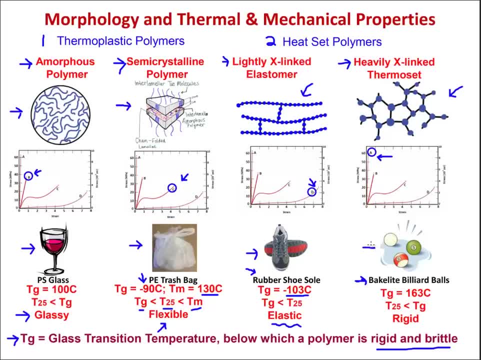 The everyday item made of bakelite we've been using is billiard balls. So the glass transition temperature of bakelite is 163 degrees Celsius. so room temperature is well below the glass transition temperature. Therefore, at room temperature bakelite and thermosets behave. 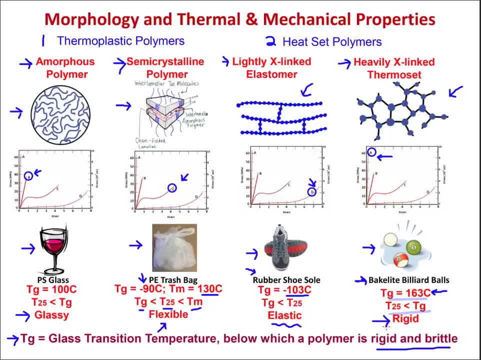 like rigid glassy solids. So there you have it, The four morphology types categorized by being thermoplastic or heat-set, just like in the concept map earlier, and along with their mechanical and thermal properties and how microstructure relates to all of that. 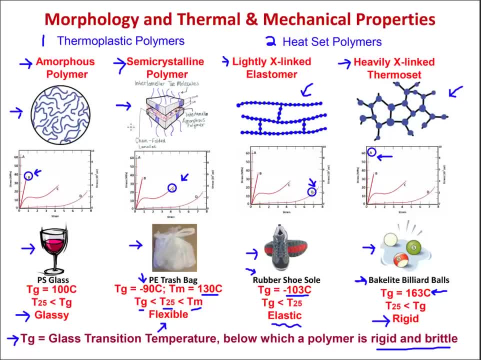 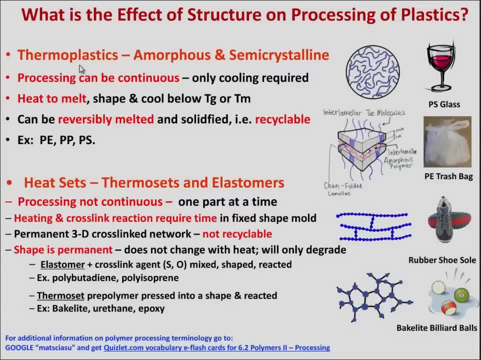 The next few slides are going to be talking about how these morphology types affect processing of these types of polymers. Now we've discussed both the mechanical and thermal properties of polymers, based off of their structure. We've also categorized them into two different categories: thermoplastic. 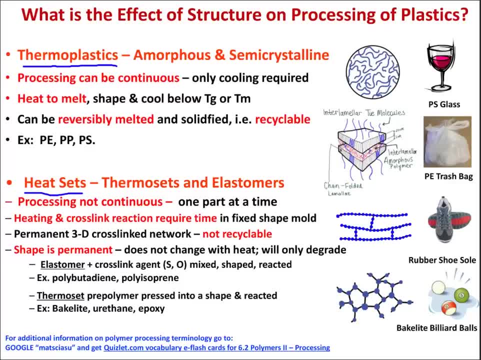 and heat-sets. We know how the structure affects the mechanical properties. That's all fine and dandy, but how does the structure affect the processing of these plastics? When I say processing, I mean methods by which we make products So like what is an example way of. 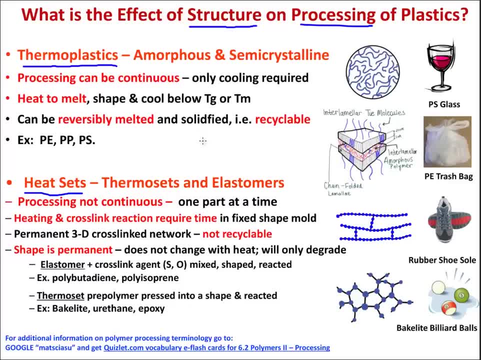 how we would make each of these four example items. The processing that is used depends on the structure. So for our thermoplastic, amorphous and semi-crystalline polymers the processing can be continuous because only cooling is required. Again, you can melt and 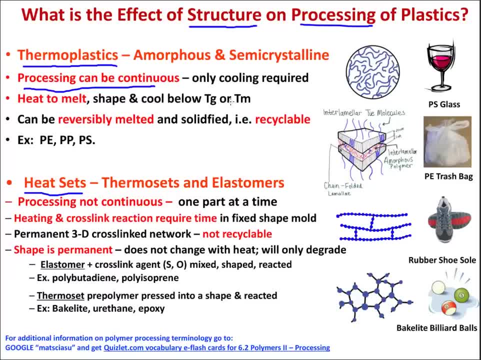 remelt and then you shape it and cool it below its T sub G or T sub M, So, as stated previously, they can be reversibly melted and solidified. So, yes, they are melt-recyclable. So, like our examples, 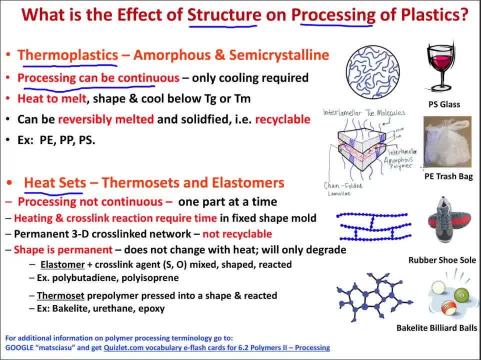 would be our polystyrene glass and our polyethylene trash bag. Now, on the other hand, we have our heat-set thermosets and elastomers. Our processing is usually not continuous. That's the big difference. You usually have to process them one. 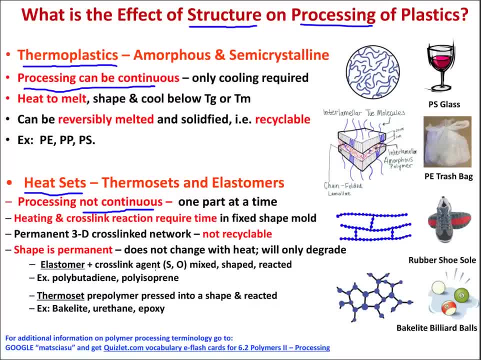 part at a time. The heating and cross-linking reaction requires time in a fixed shape and mold because of that, And the 3D cross-link network is totally permanent. Therefore they are not melt-recyclable. Here are two example ways of 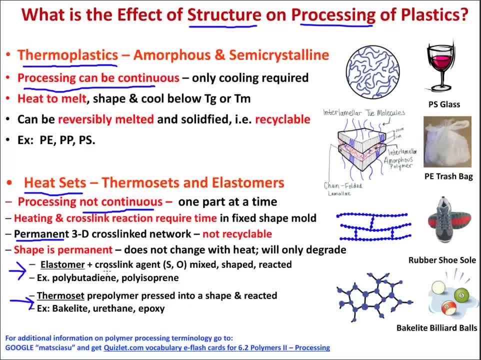 methods of the cross-linking. The elastomer is put in with a cross-linking agent. It's mixed, shaped and reacted. So this would be like our rubber- polybutadiene, our rubber here For thermosets, the prepolymer. 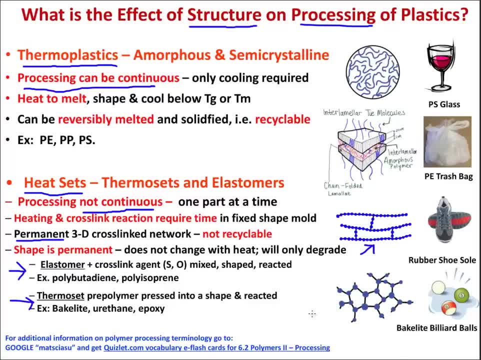 is pressed into a shape and then reacted. So again, this would be like our bakelite heat thermoset. Now that we have an idea of how the structure affects the processing, the next slide will be going through example processing techniques that could have been. 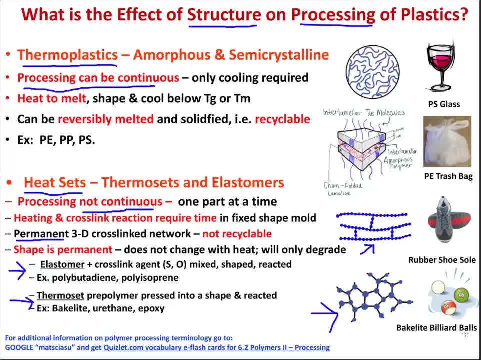 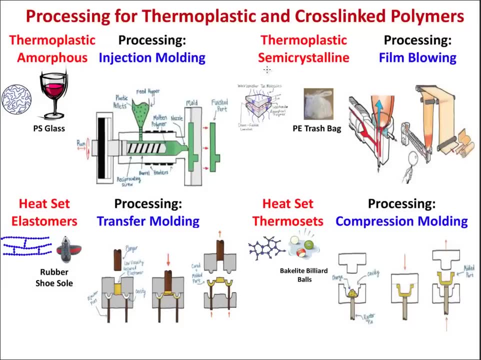 used to make our four everyday example items. Also, I have included a link to MatSciASU's Quizletcom, which allows you to study vocabulary flashcards for polymers Preparation. Previously we've discussed the main difference between the processing of thermoplastic and 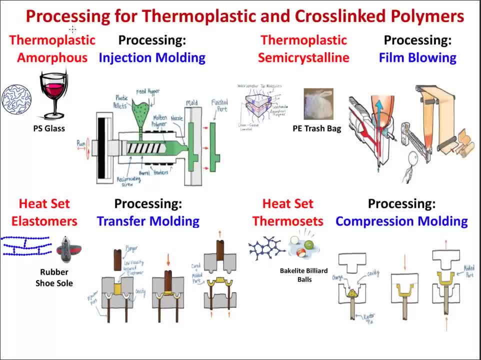 heat-set polymers. Thermoplastic polymers can be processed continuously, but heat-set polymers cannot usually be processed continuously because the cross-linking reaction requires time. They need to be cured. So, while keeping that in mind, I'm going to go through. 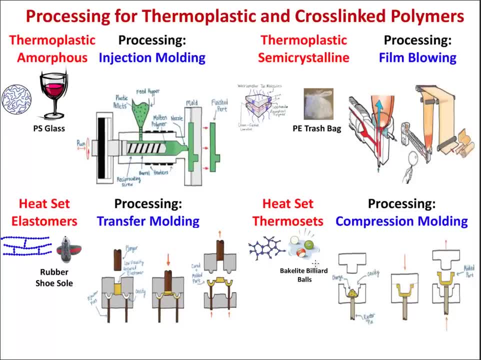 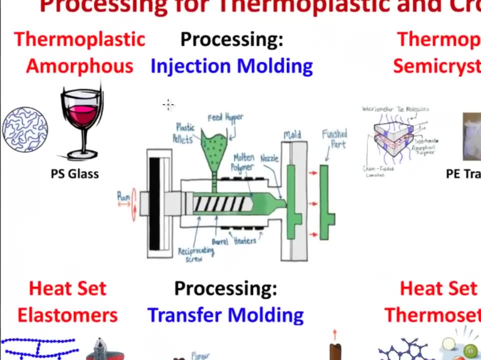 four example processing methods, one for each morphology type that was most likely used to make the everyday polymer item representative of that type. So, starting with our thermoplastic amorphous polystyrene drinking glass, The processing used was most likely. 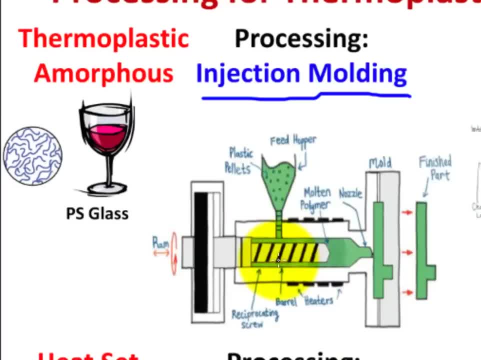 injection molding. As you can see in the diagram here, the molten polymer gets pushed through the nozzle into the mold and then a finished part pops out on the other side. This is continuous and very fast, So it would be perfect to make a very 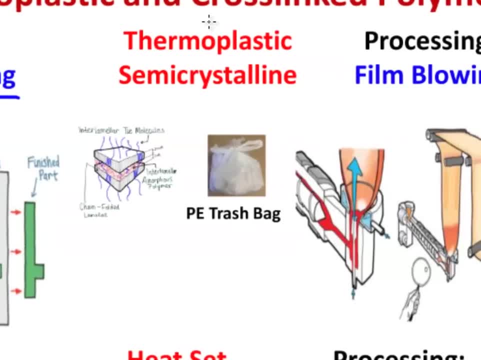 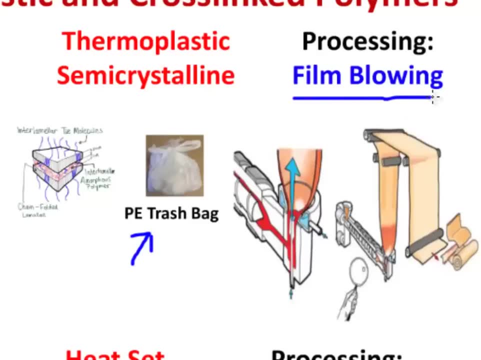 inexpensive drinking glass. For the thermoplastic semi-crystalline polyethylene trash bag, the processing most likely used was film blowing. So basically what happens in film blowing is that this molten polymer here has air blown through it, so it is expanded. 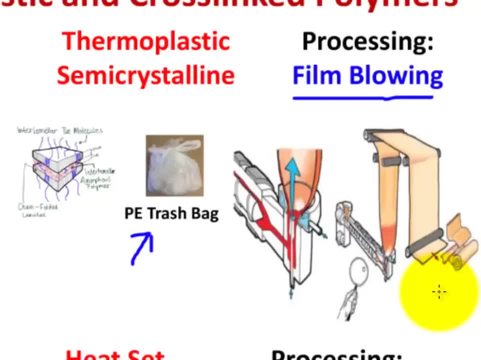 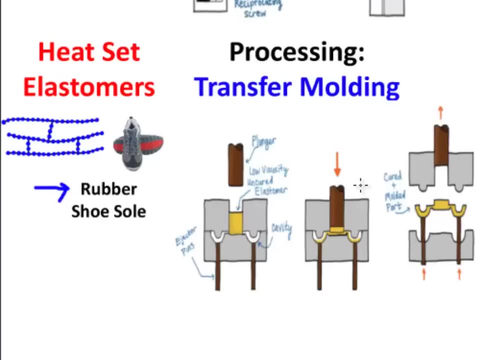 like so along the sides and becomes a very thin film And it's collected in rollers and sheets like so. This is also a continuous processing method For our heat-set elastomer rubber shoe sole. the processing used was most likely transfer molding- Basically what happens. 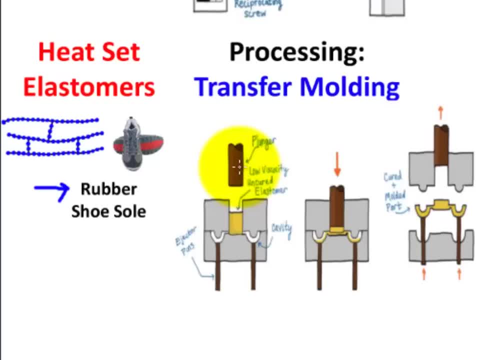 is. you have this uncured elastomer here. This plunger comes down and pushes this polymer into this mold. The elastomer waits inside the mold for a little bit and then the finished part is ejected through these pins at the bottom. So as you can see this. 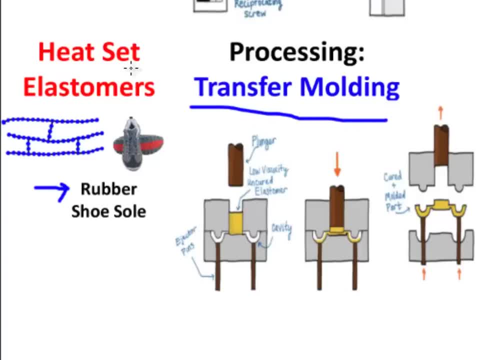 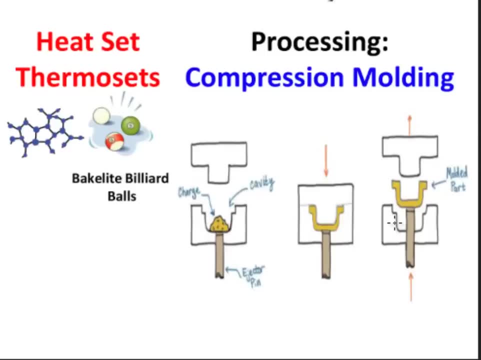 process. transfer molding gives time for the elastomer to be cured in the mold. Finally, for our heat-set thermoset bakelite billiard molds, it was most likely made through compression molding. It's very similar to transfer molding, but basically the uncured. 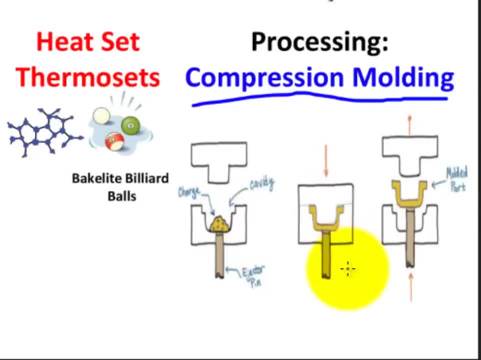 polymer begins inside the mold, then it is compressed into this molded shape and then ejected out. So again, the heat-set thermoset polymer has time to be cured inside of this mold, right here. So there you have it, We've gone. 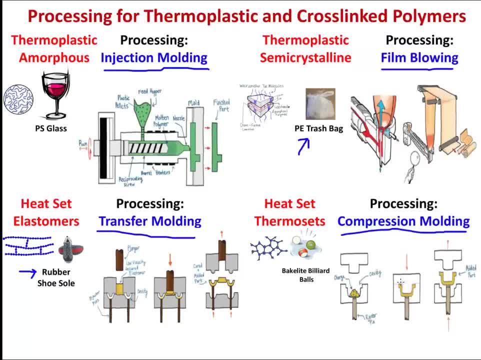 all the way through from how the microstructure affects the mechanical properties, talked about the thermal properties of the glass, transition temperature, and we've now gone through and shown how different example everyday items are processed based off of their microstructure. This is all great, but how exactly? 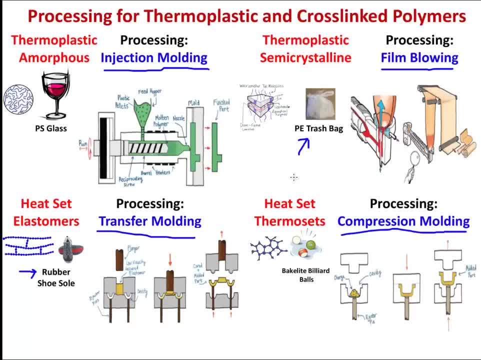 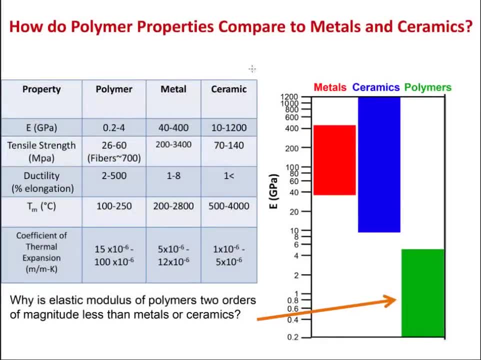 do polymers compare to the other material classes like ceramics and metals? And that is what is going to be addressed in the next slide. We've spent all this time talking about polymers, building up what our definition of a polymer is through how we describe the molecules. 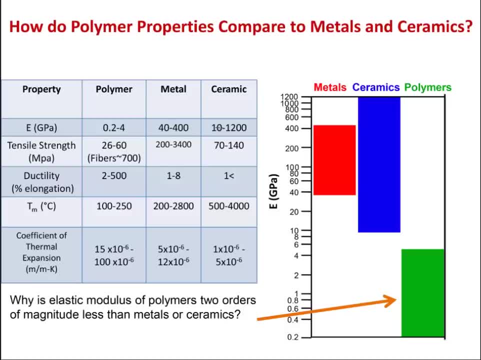 themselves, to how we describe how the molecules create different types of morphologies, how we classify, how we can determine mechanical properties from the morphologies, how we can determine processing from the morphologies. This slide shows you how do polymers like polyethylene 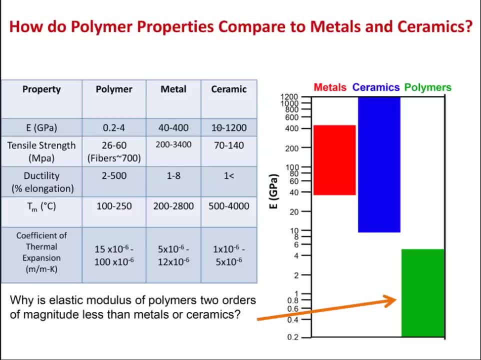 compare to metals and ceramics. So you have a full picture of what polymers are. We have different properties listed here: Polymers, metals and ceramics. We can see that in general, polymers have lower elastic moduli than metals or ceramics. They also have 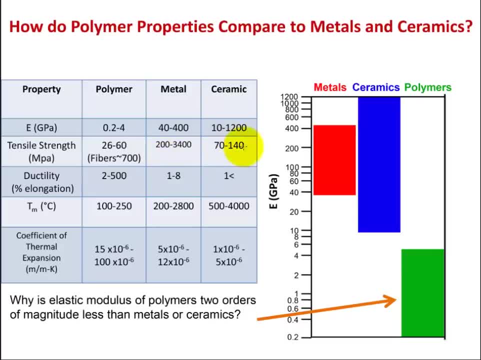 lower tensile strength, like orders of magnitude lower- than metals and ceramics. They have much more ductility, though. They have lower melting temperatures than metals and ceramics and they have generally higher coefficients of thermal expansion. So this diagram here serves to show you the range of elastic. 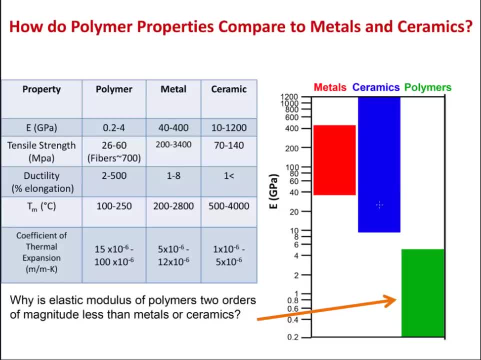 moduli in gigapascals for the three material classes. So this red bar represents metals, blue is ceramics and then green would be polymers, which are way down here. So why is the elastic modulus of unoriented polymers two orders of magnitude?